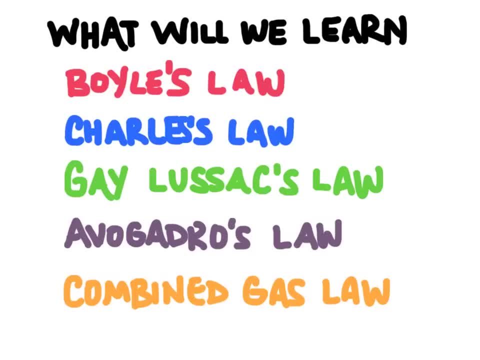 From an initial set of conditions to a change set of conditions And each of the laws is going to compare two variables, except for the Combined Gas Law, All the other ones, we'll just look at two of those variables we mentioned right up here at a time. 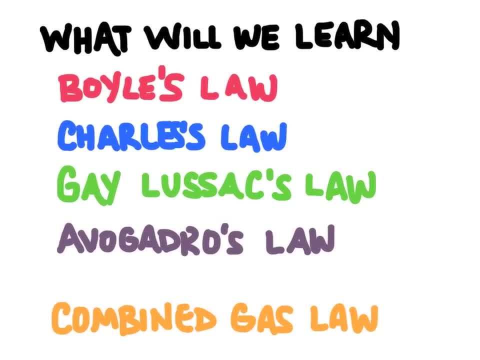 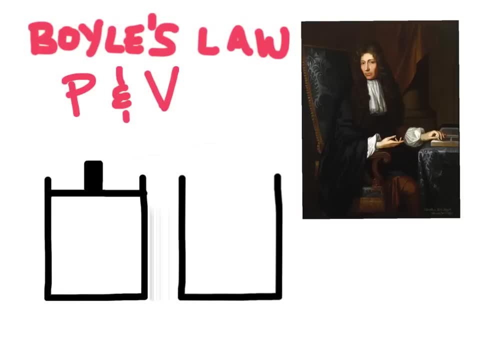 And the other ones will remain constant. So let's start with Boyle's Law. Boyle's Law relates pressure and volume, And it was published by Robert Boyle in the late 1600s. Boyle said that when the pressure of a gas increases, the volume of a gas decreases. 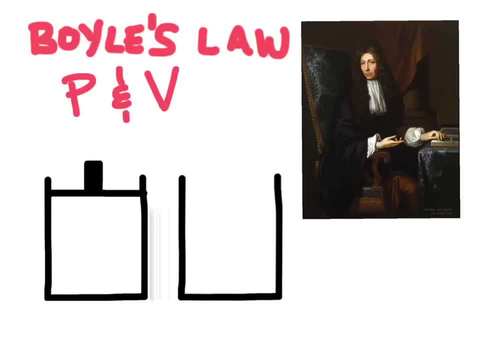 As long as the temperature and the amount of gas are held constant. So if you can imagine, in this container- this first one right here- we just had a bunch of gas particles And this little bit of weight right here was being suspended by those gas particles. 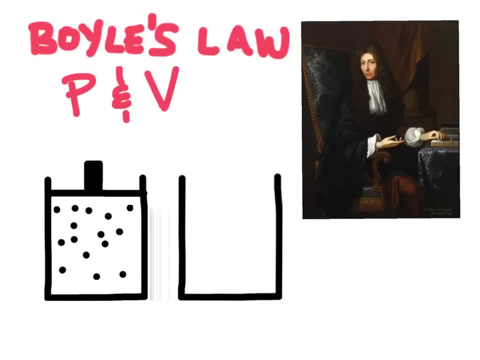 And so if we increase the weight to increase the pressure over here in the second one, So if we added a whole bunch more weight on top, We would decrease the volume because the pressure went up and so the volume would go down. 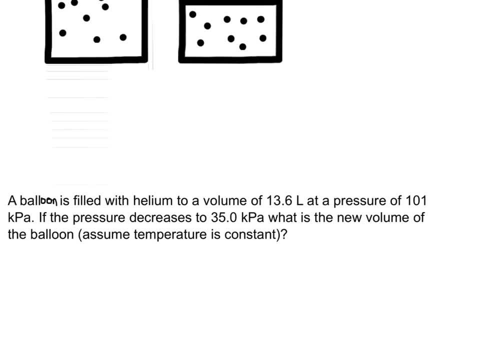 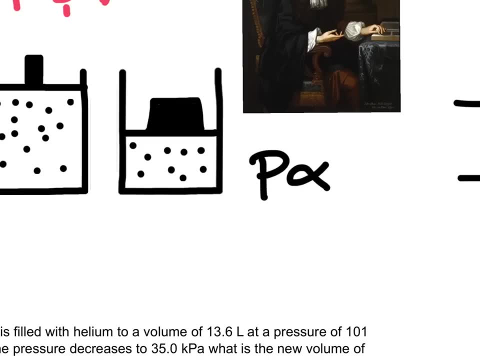 Now, mathematically, the relationship will be inverse, And so we could say that pressure is going to be proportional to the inverse of the volume, And this is just a fancy way to say. as pressure goes up, volume goes down. 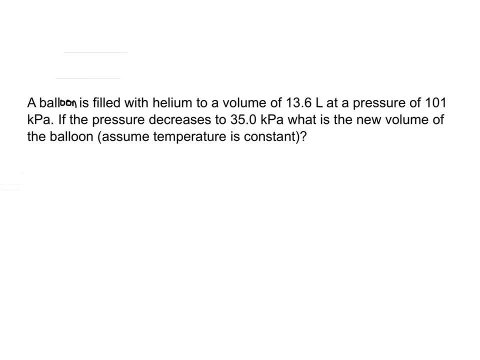 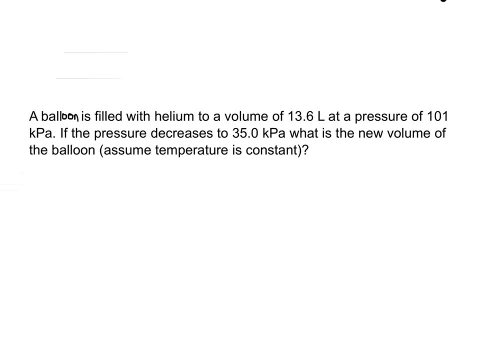 Now, when we're looking at a problem, We're going to solve this problem. We're going to solve this problem in a minute. We're going to use the mathematical relationship for Boyle's Law. It's going to compare an initial set of conditions to a changed set of conditions. 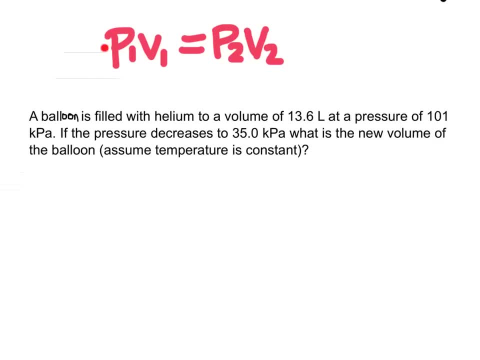 And so here's how that equation would look. This left side of the equation represents the initial set of conditions, And so I have an initial pressure: I'm calling that P1.. An initial volume: I'm calling that V1.. 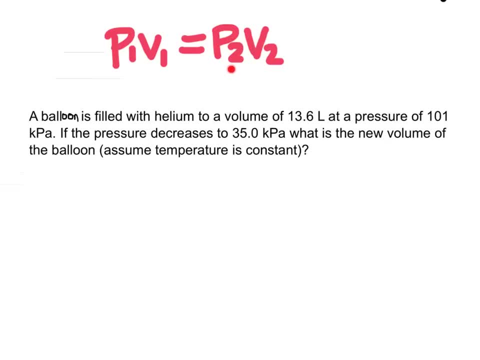 And then over here is our changed set of conditions. So the pressure, the new pressure will be P2.. And the new volume will be V2.. So what we're going to do in this problem Is: we'll read through it. 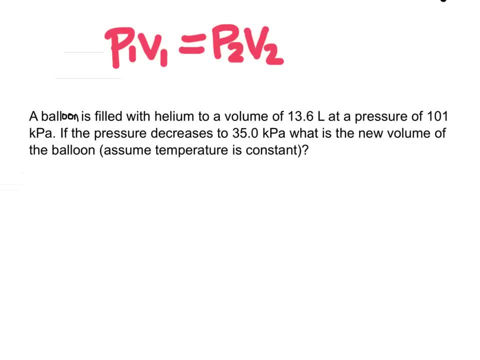 And we'll underline the information that is given to us And then underline what the question is asking for. It says that a balloon is filled with helium to a volume of 13.6 liters At a pressure of 101 kilopascals. 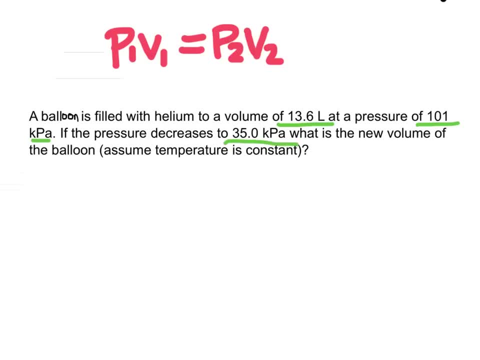 If the pressure is decreased to 35 kilopascals, What is the new volume? And we can see assume temperature is constant. So I can see that there's an initial set of conditions. The balloon is filled with helium to an initial volume. 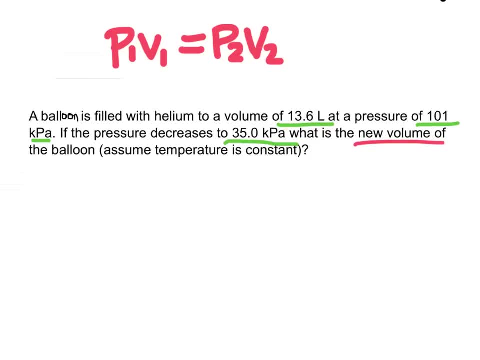 That's V1. And an initial pressure, That's right here: 101 kilopascals, That's P1. And then we change it, We decrease the pressure. This is P2. And we're going to solve for V2.. 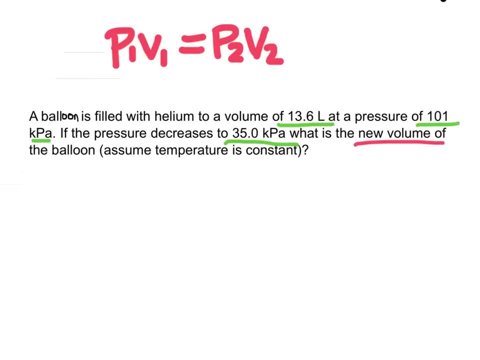 What I like to do is list all of the data that I have And assign it the correct variable before I start solving the problem, And so here is all the information listed, And I'm going to use this equation right here. I'm going to solve for V2.. 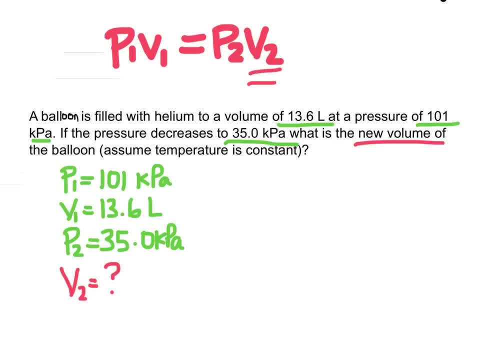 That's what I'm solving for. So I'm going to rearrange the equation by dividing both sides by P2.. It's going to cancel P2 on this side and move it over here, And I'll rewrite that down here. So I have: V2 is equal to P1 times V1 over P2.. 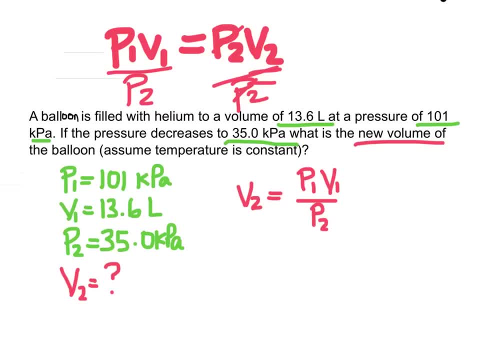 So we'll go ahead and plug in all of our known information, And it's just a matter of plugging this into our calculator, And we'll end up with a new volume of 39.2 liters. And so that is Boyle's Law. 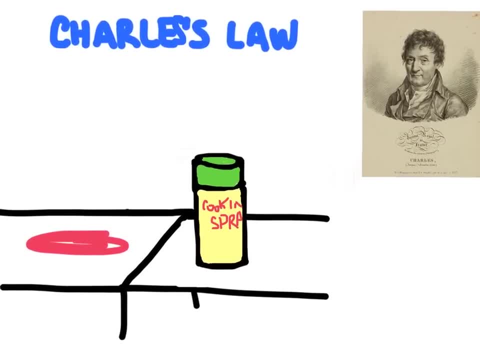 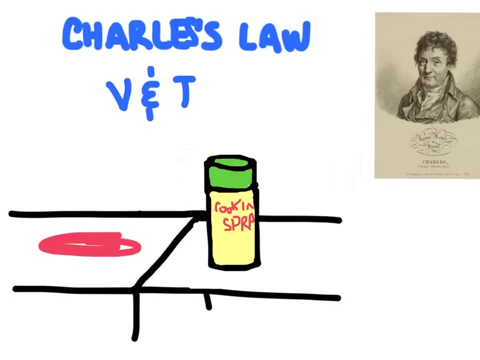 Let's move on to Charles' Law. Charles' Law is going to relate volume and temperature, And this law was formulated by Jacques Charles. He was a French chemist And this was in the late 1700s. Charles said that as the temperature of a gas increases, the volume of the gas will also increase. 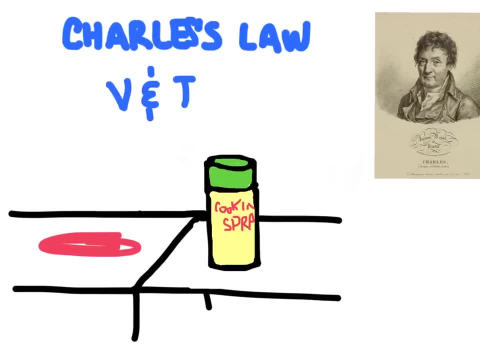 And that's if pressure and amount of gas are held constant. Now, this is a direct relationship And don't try this at home, But this is the example I thought of here. If you were to accidentally take your cooking spray and set that onto a hot burner. 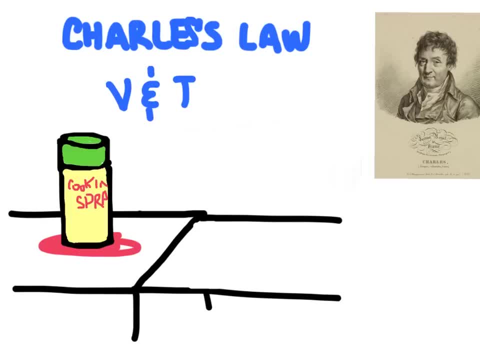 the temperature of the gas inside would start going up And as the temperature increased, the gas would start expanding, attempting to increase the volume of a container. Now, eventually it would rupture the can and allow for that increase in volume. Now, mathematically, this relationship would look like this: 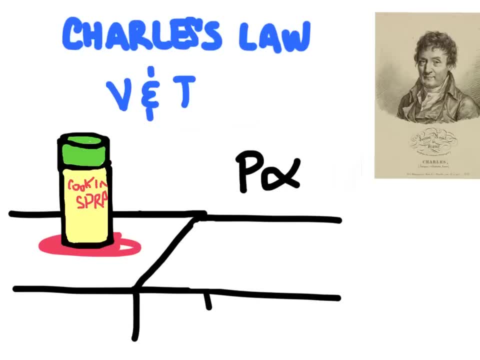 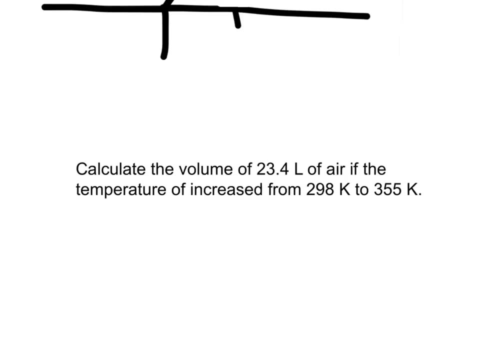 P is proportional to V, Or in other words, direct relationship. so as pressure increases, volume increases. If we were comparing or looking at a problem here, and we're comparing an initial set of conditions to a changed set of conditions, the equation would look like this: 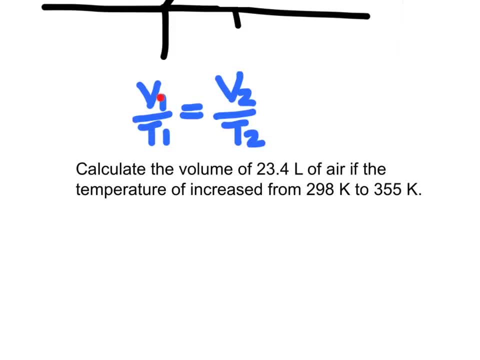 And so we have our initial set of conditions here, of an initial volume and temperature and a changed volume and temperature. So let's solve this problem, And we'll do this the same way as Boyle's Law. I'm going to read through it and underline the given information. 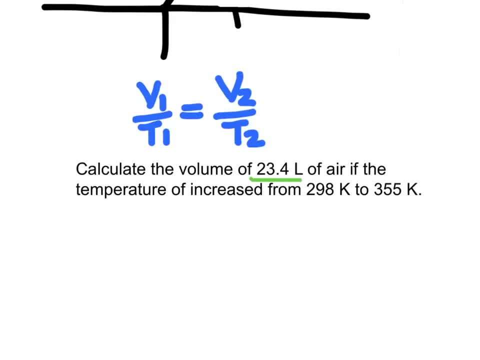 It says: Calculate the volume of 23.4 liters of air if the temperature was increased from 298 Kelvin to 355 Kelvin, And we're solving for volume in this case. I'm going to go ahead and list the information that I know. 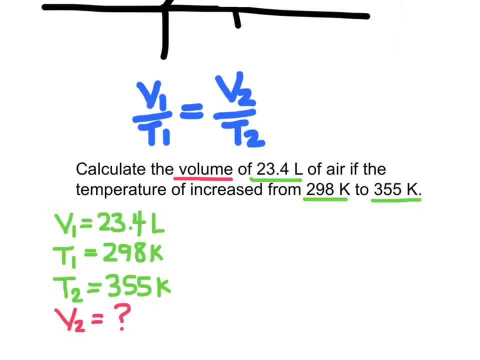 So I know the initial volume when it started out here. That's V1.. And I know that the temperature started at 298.. That's my T1. And it increased to 355.. So that's T2.. And so I'm solving for V2.. 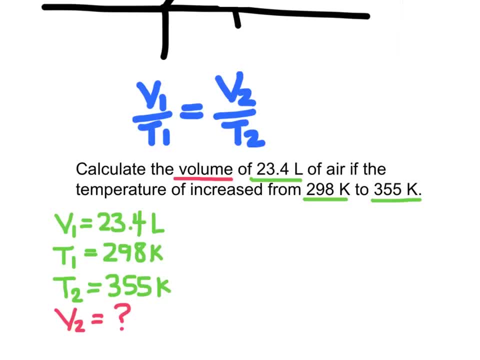 I'm going to rearrange this equation that I have up here by moving T2 up to the other side, And I'm going to end up with V1 times T2 over T1. It's going to be equal to V2.. So now I can plug in all of my known data. 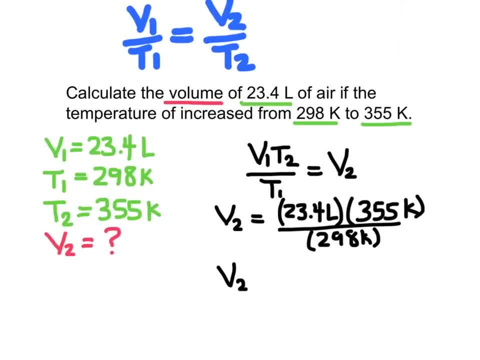 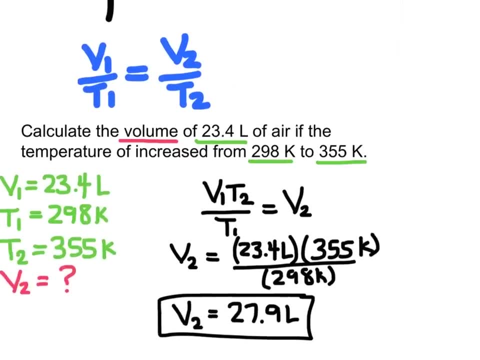 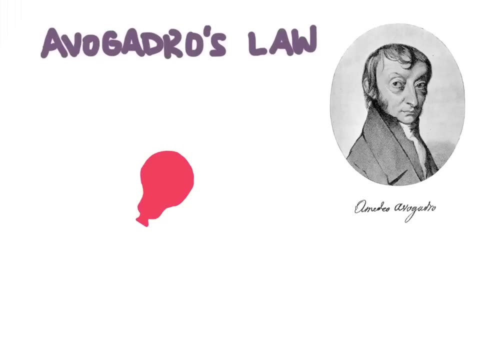 And I'll end up with a new volume That's equal to 27.9.. And so that's Charles' Law. The next one is called Avogadro's Law, And this is going to relate the amount of gas and volume. 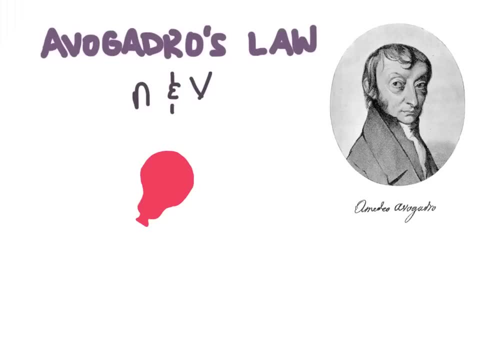 And this law was formulated by Amadeo Avogadro, who formulated this in the early 1800s, And the law is probably the most intuitive of the gas laws. It says that as you increase the amount of a gas, the volume of a gas will also increase. 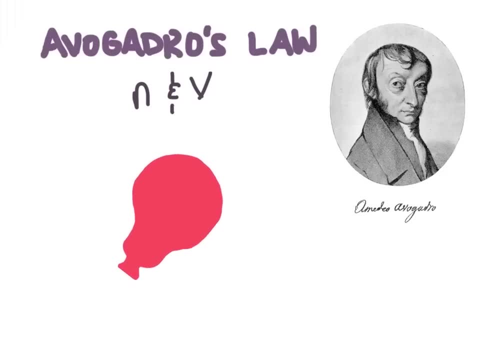 And so it's just as you blow more air into a balloon, the balloon will get bigger and bigger and bigger. Now, mathematically, the relationship is going to be a direct relationship, So the number of moles of gas is going to be increasing. 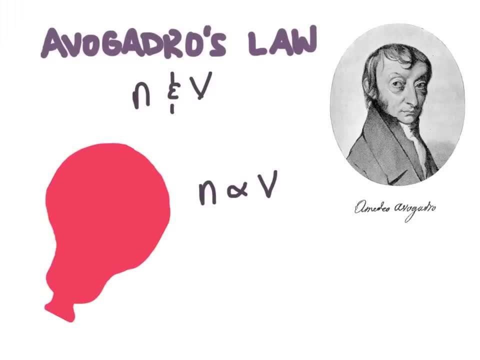 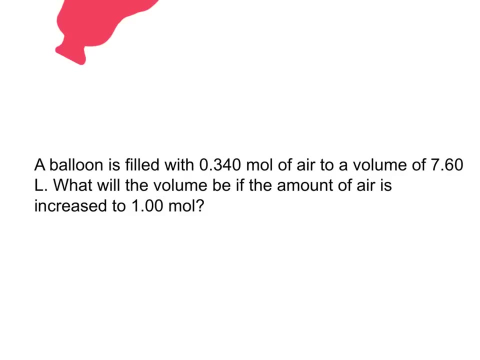 That means the volume will also be increasing. So let's look at an example of a problem once again, And we'll start off with that equation that relates an initial set of conditions to a changed set of conditions. So we have our volumes and our amounts. 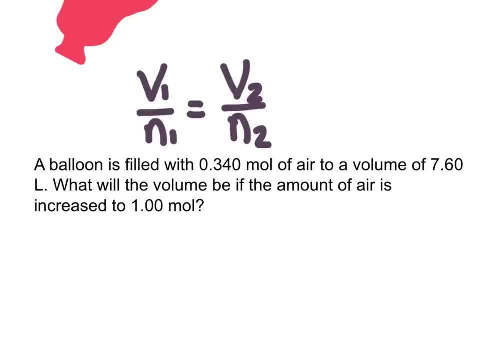 And we use the letter N to signify number of moles. Let's read this problem and I'll underline once again the given information. It says a balloon is filled with 0.34 moles of air to a volume of 7.6 liters. 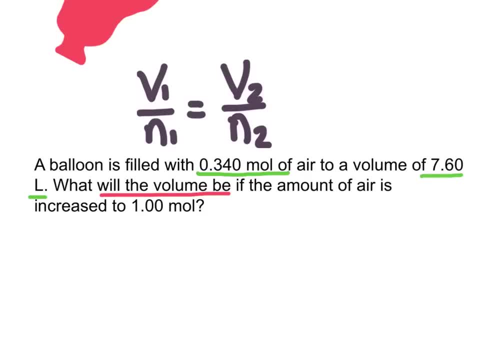 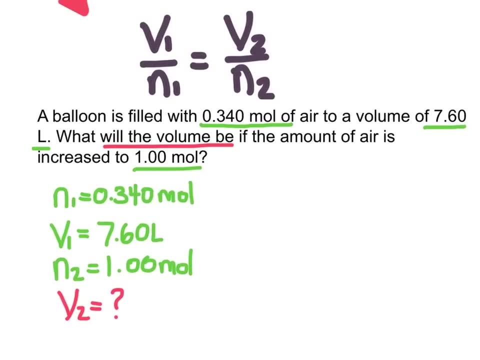 What will the volume be if the amount of air is increased to 1 mole? Let's go ahead and list the data, And then we can rearrange this equation by moving N2 up And we'll get V1 times N2 over N1 be equal to V2.. 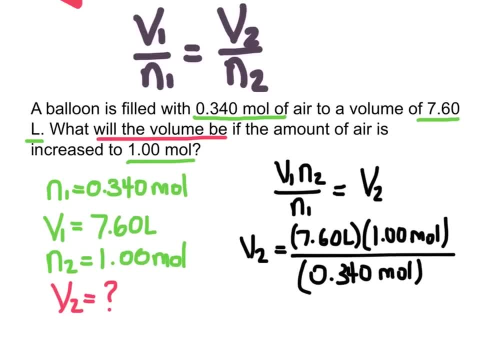 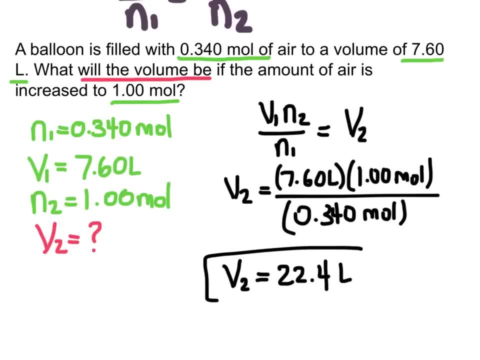 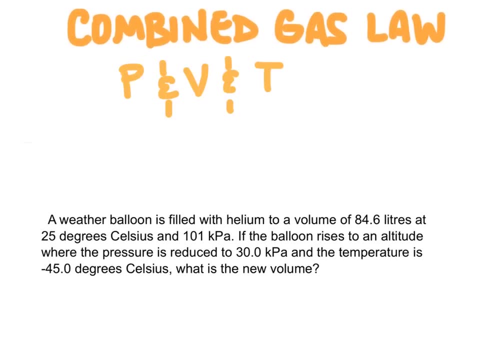 And I can go ahead and plug in my known information, And we end up with a new volume that's equal to 22.4 liters. Alright, one last law, And it is called The Combined Gas Law, And this law is going to actually combine Boyle's Law, Charles' Law and Gay-Lussac's Law. 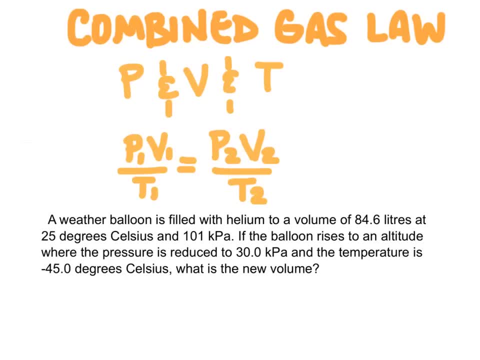 So it looks at pressure, volume and temperature, And so this is what the equation looks like, And this allows for actually two things to change. In the previous problems, only one variable was changing. We're calculating another variable. In this problem, we're actually going to have two of the variables change. 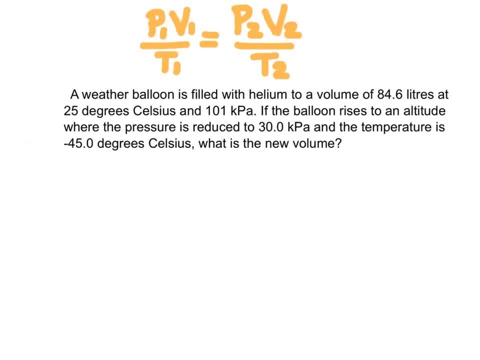 So let's read it. It says: a weather balloon is filled with helium to a volume of 84.6 liters At 25 degrees Celsius and 101 kilopascals If the balloon rises to an altitude where the pressure is reduced to 30 kilopascals. 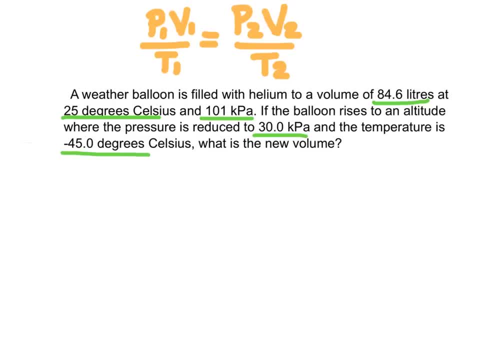 And the temperature is negative 45 degrees Celsius. What is the new volume? I'm going to go ahead and list all of that known data, And there's everything there. What I need to do is check all the SI units, Make sure everything's in standard units.